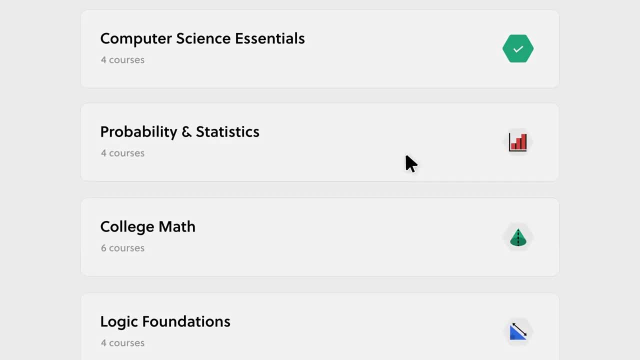 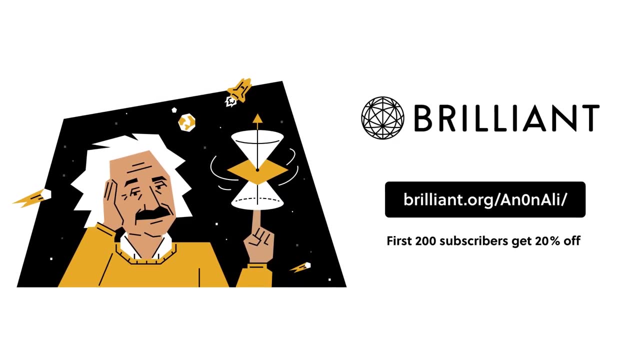 aspiring hacker looking to clarify your concepts, or a professional looking to upskill, you can try everything Brilliant has to offer free for 30 days and if you sign up using Brilliantorg Ali, the first 200 of you will get a 20% discount on Brilliant's annual premium subscription. 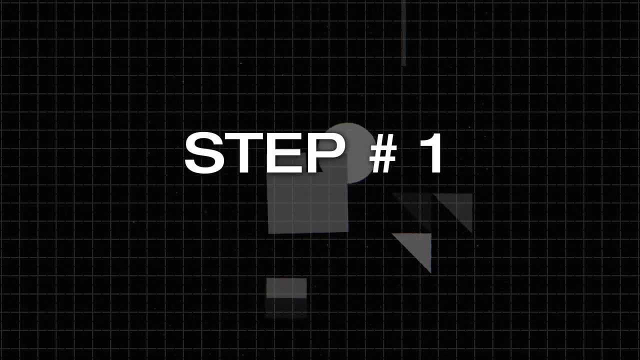 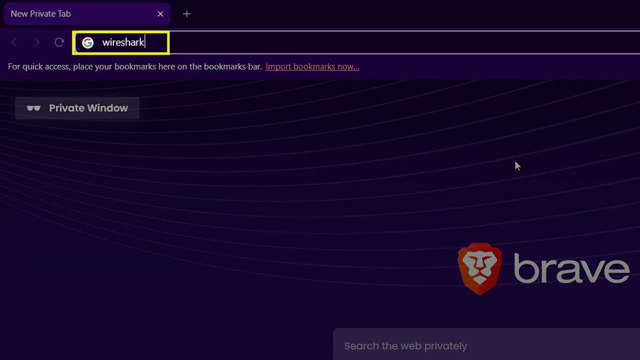 Thanks for listening. let's get back to the video. Step number one: download and install Wireshark. Okay, so before we dive into what network analysis means and how Wireshark is used, what I want you to do is head over to its official website and download it according. 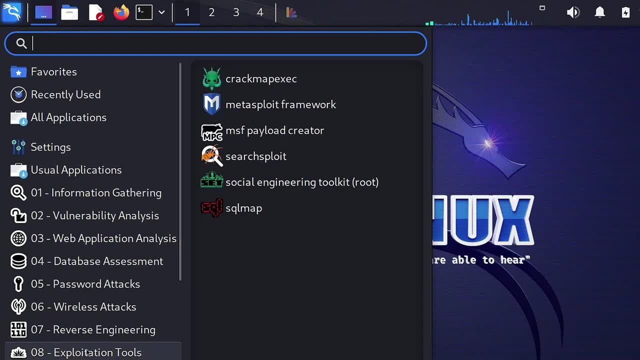 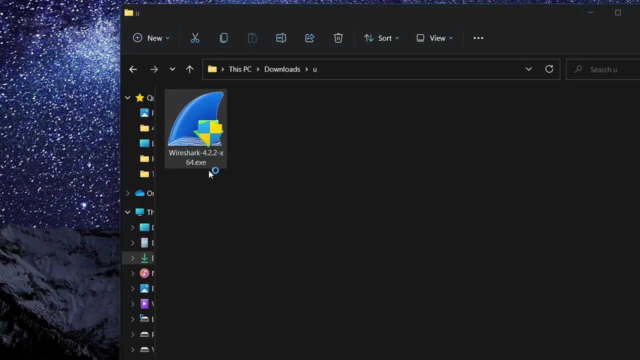 to your main operating system like this: If you're using Kali Linux, you can go ahead and skip this step as it comes pre-installed on it, but for other operating systems, once you've downloaded it, open it and install it. During the installation, you'll be prompted to. 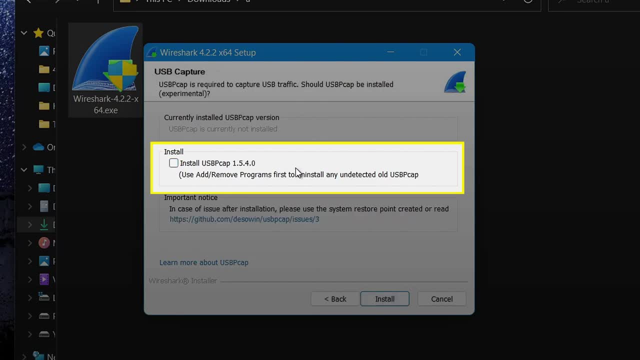 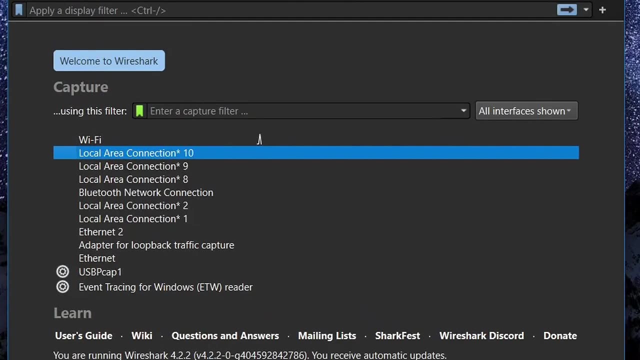 install these additional packages called npcap and usbpcap to ensure everything works properly, so make sure to include them as well. Once installed, you can launch Wireshark, to be greeted with a welcome page like this, and from here you can basically select the network. 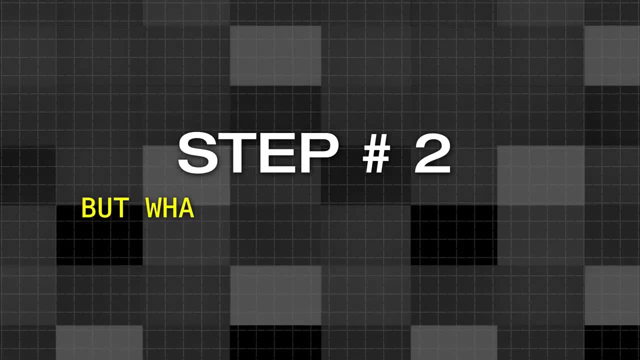 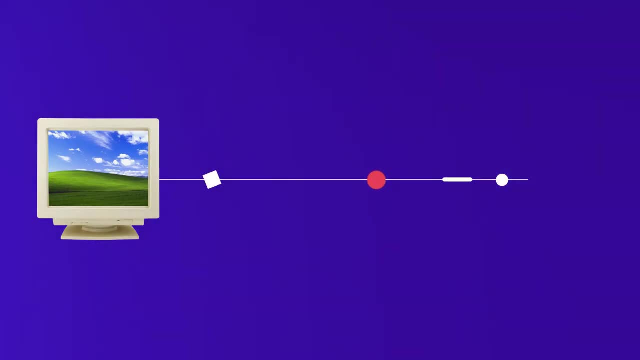 interface card that you want to analyze the traffic from Step number two, but what is traffic analysis? Okay, so when I say the term analyzing the traffic, what I essentially mean is opening the packets or letters that are being sent from one device to another over a network and seeing 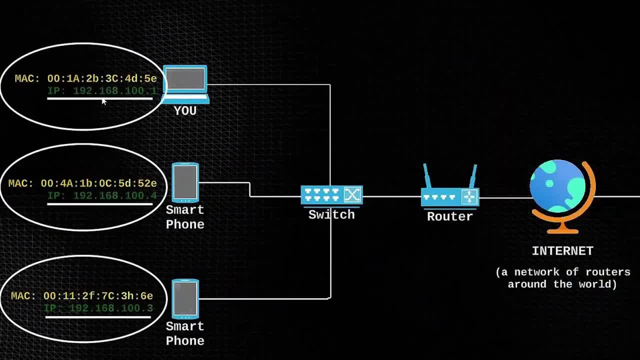 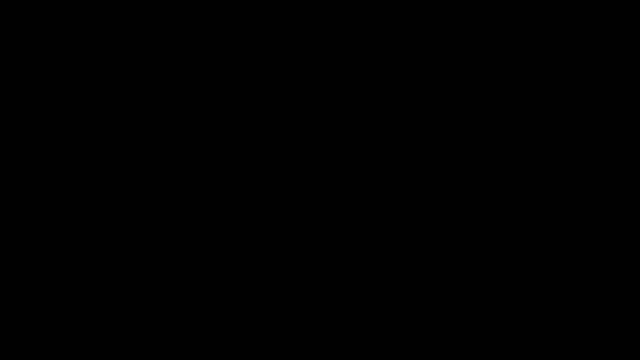 exactly what each one says. Now, if you're not sure about what a packet is or how computer networks are, then checking out this video first, as it will make it easier for you to grasp everything that I'll be talking about here. but for now, just know that if I open up a website on my browser, 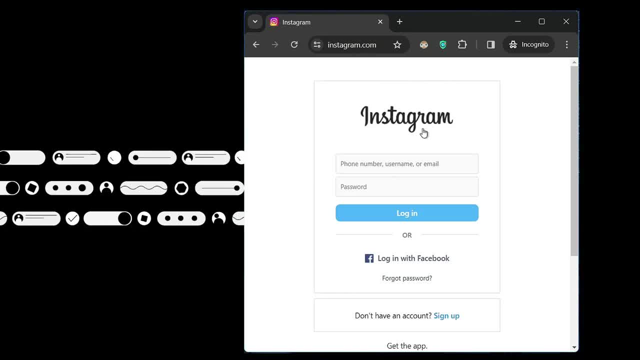 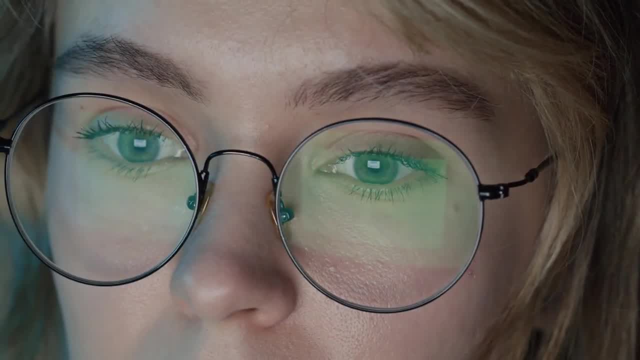 and want to see what communication is happening between my computer and the web server of this website behind the scenes. I can do that by using Wireshark, and this is what network analysis essentially means. Now, the reason why hackers need to be skilled at this involves several factors. 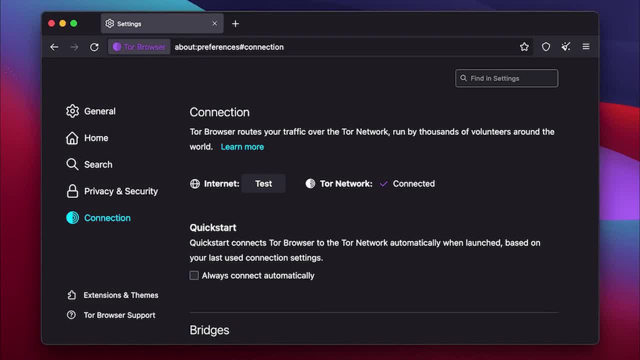 which I can't go over in this video, but just to name a few. it may help them in using Wireshark with Tor to ensure everything is going right and their anonymity isn't being compromised or identify multiple vulnerabilities in the network. So if you're using Wireshark, you can. 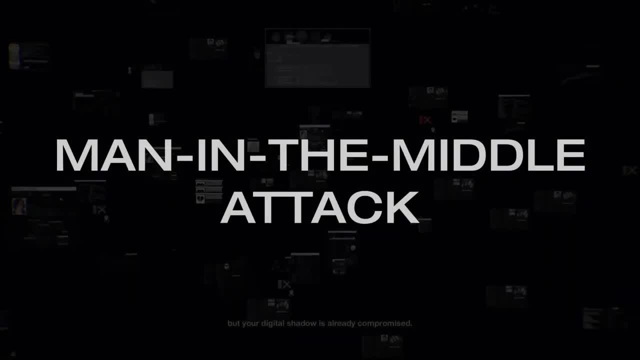 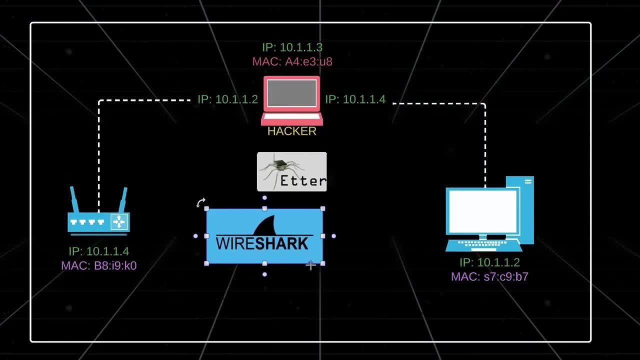 use Tor to identify multiple vulnerabilities within a network before attacking it, and even perform things like a man in the middle attack, where they essentially place themselves between two communicating devices using a tool like Ettercap and then analyze someone else's traffic with Wireshark to see what websites they're visiting or capture sensitive information. 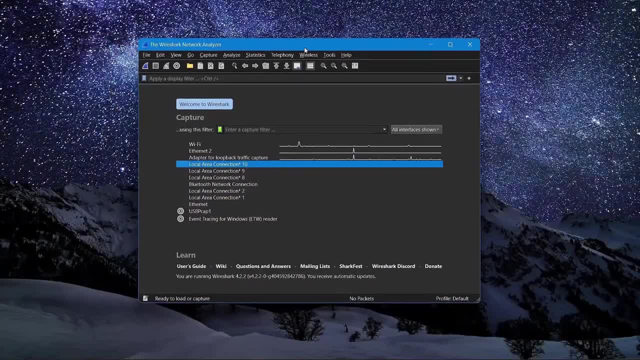 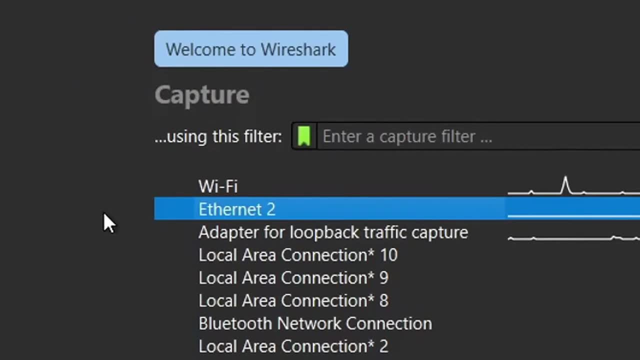 like their passwords. Step number three: Wireshark interface. Okay, so depending on the network interface cards you have available on your computer, this page might look a little different than mine, but essentially what you want to do here is select the network interface card that. 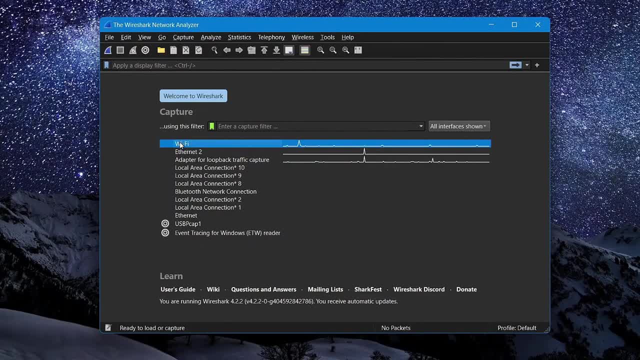 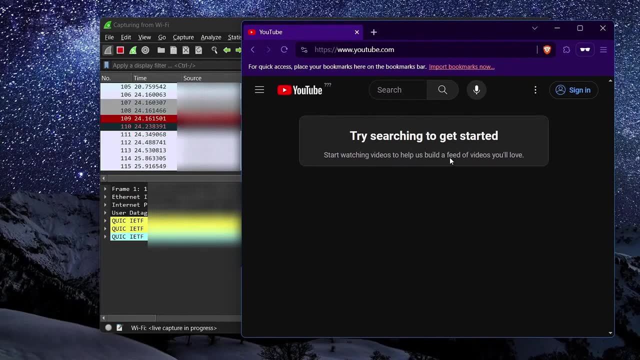 you're connected to the internet with and want to capture packets from. Since I'm connected to WiFi, I'm going to choose this option by double clicking on it like this. Next, Wireshark will start doing its magic and begin capturing the packets that are being sent from. 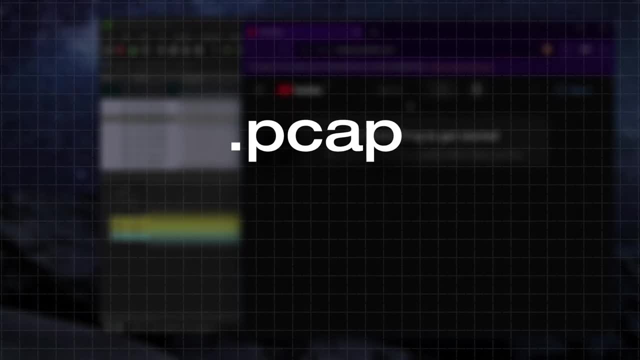 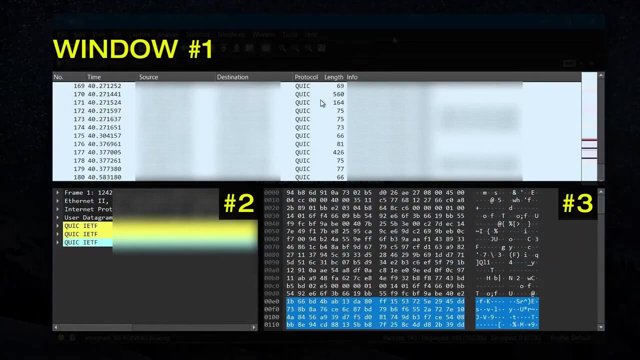 our browser to this web server over the internet and then save them into a pcap format, which is a standard file format for capturing packets. Now if we stop capturing the packets by clicking on this red button here and then assign numbers to all the windows we see within Wireshark? 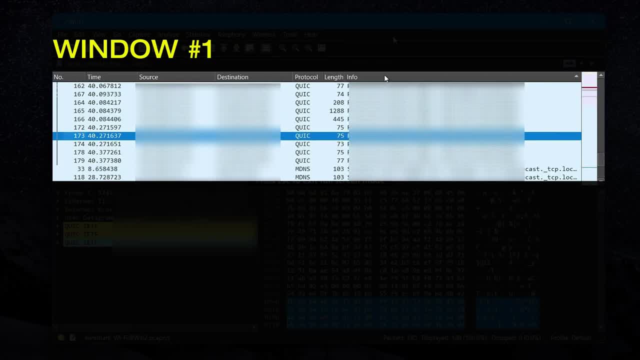 the top window, which is labeled as number one, is called the packet list pane, and this is where all the packets that Wireshark is capturing are shown in real time. Here the source IP address is the device sending the packets, and the destination IP address is 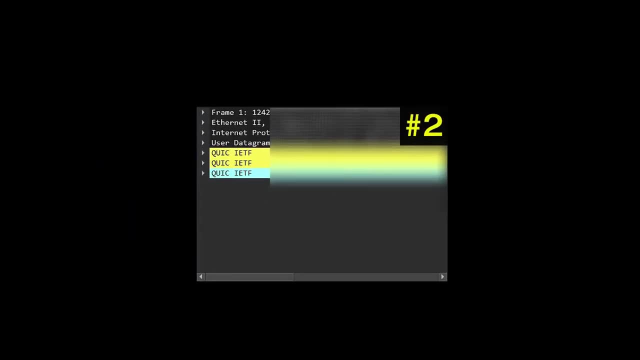 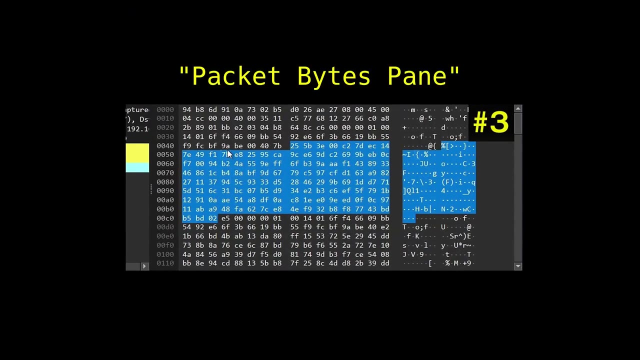 the device receiving them. The bottom left window, labeled as number two, is called the packet details pane and it shows us information on a selected packet from window number one, Whereas the bottom right window is known as the packet bytes pane and it provides a quick way. 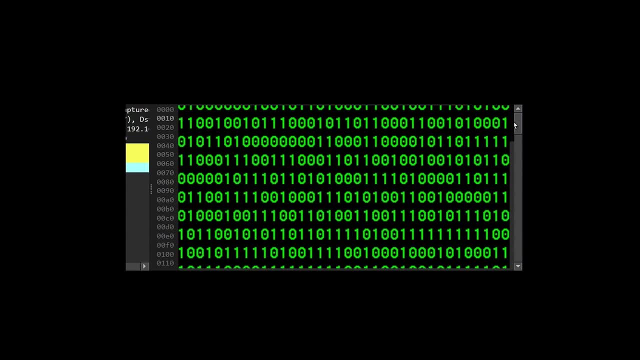 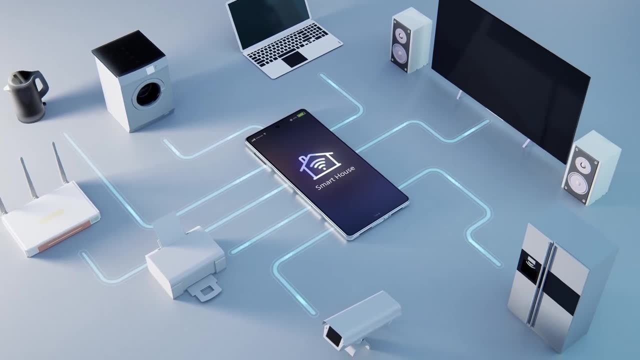 to see what a payload says in a human readable form, rather than showing the binary representation of data. Step number four: creating filters. Since modern operating systems constantly send and receive data in the background, without any user interaction, Wireshark starts capturing packets the moment you launch it, and so, if we want to focus solely on some specific packets, 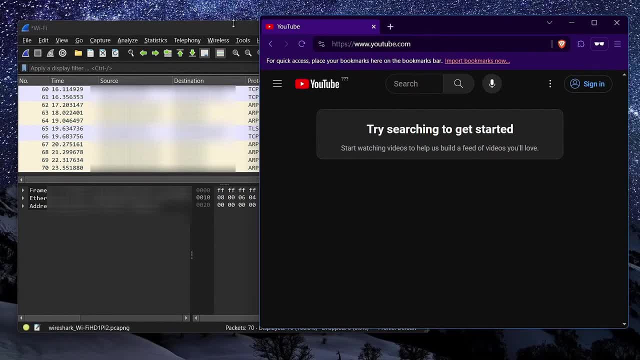 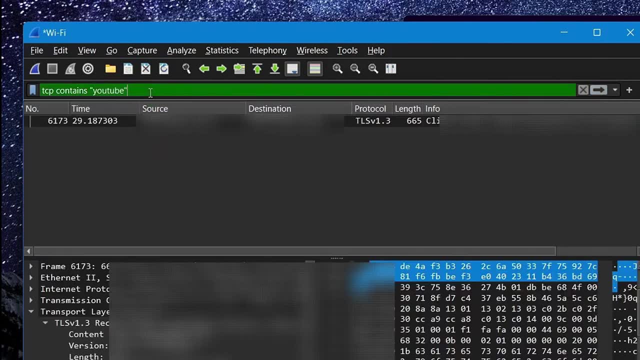 like the ones we just saw. we can do that. So if I input a filter called TCP contains and then specify YouTube like this, you can see that it has shown me one packet that it captured when I searched for YouTube on my browser. 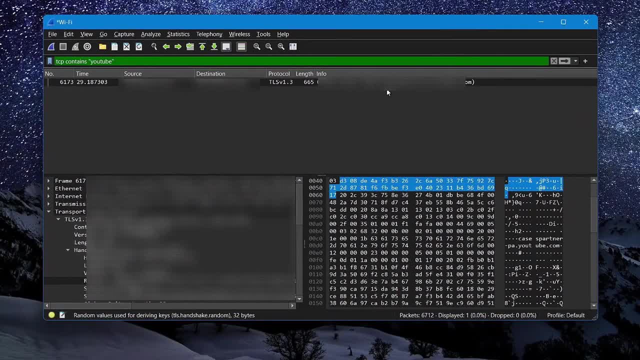 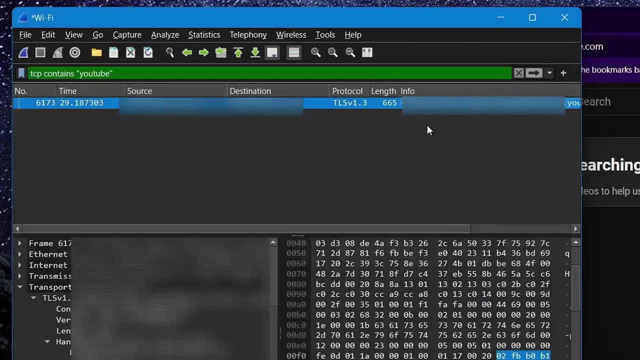 and to explore a range of other filters and operators that can be used to search for packets, just like this. you can download a PDF that I prepared by clicking on the link in the description down below, Step number five, following a stream. Okay, so, once you've identified the packet that you're interested in, 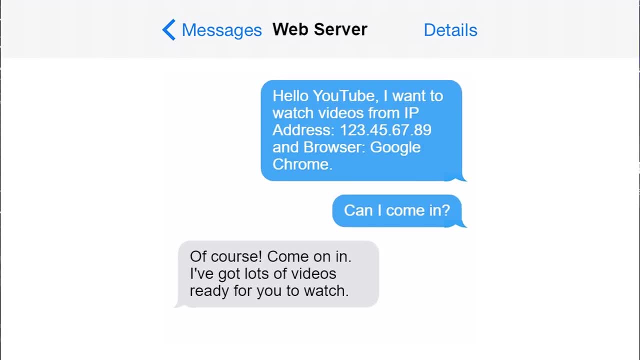 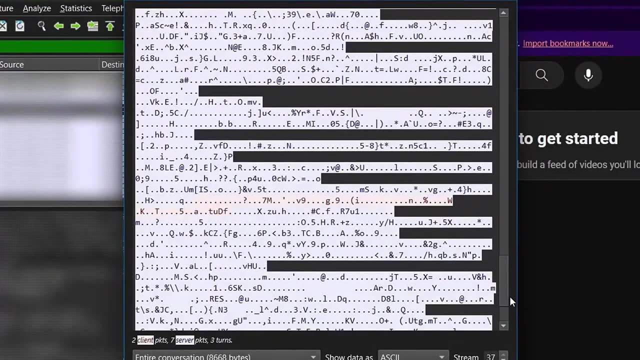 and want Wireshark to open a new tab showing all the communication between your computer and the web server of a specific IP address. what you can do is simply right click on the packet and then select follow TCP stream. like this. Now the reason why you can't understand. 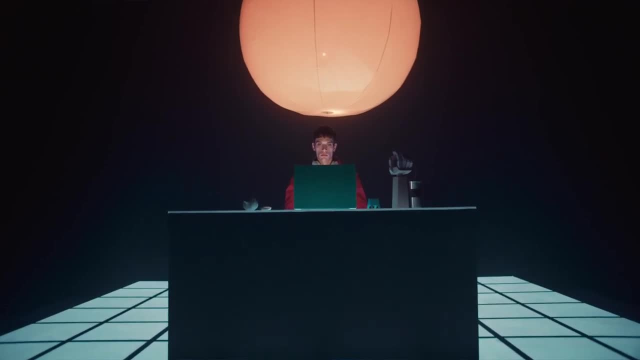 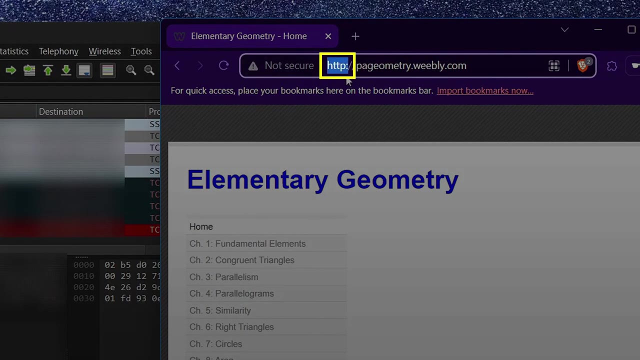 any of this is because it's encrypted by TLS encryption, which acts as a way to protect the contents of a web page from hackers when they're performing things like a man in the middle attack. but if you were testing it on a website that used HTTP in its URL rather than using HTTPS? 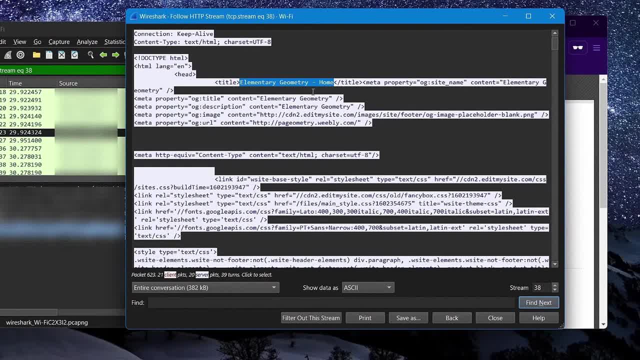 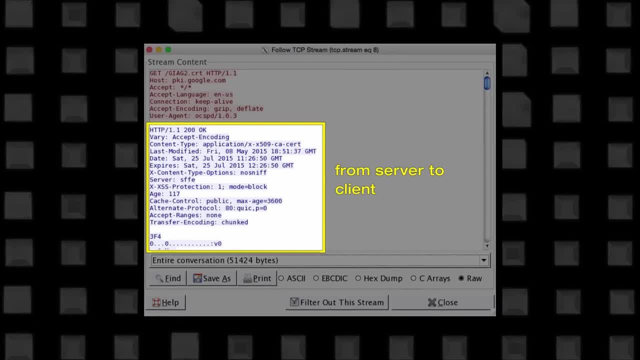 what you would get is all the communication in plain text like this, and this is the vulnerability that hackers take advantage of. Now all the requests sent here from our computer will be, and all the responses received from the web server will be shown in blue.